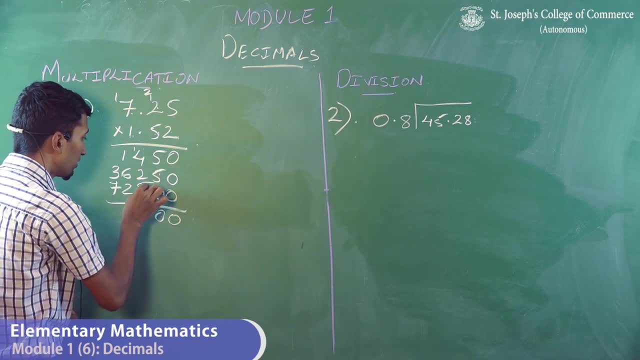 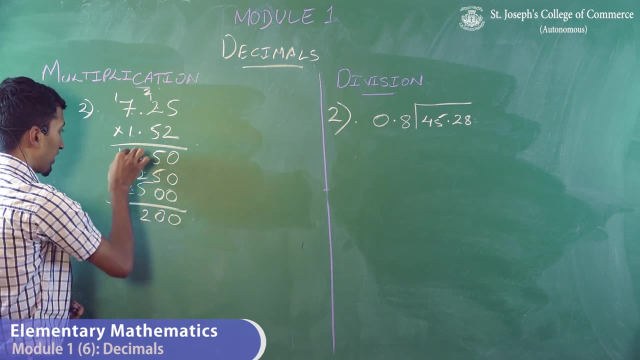 0, 5 plus 5, 10, 0 carry 1.. 5 plus 4, 9 plus 1, 10 plus 2, 12 carry 1.. 6,, 7,, 8, 9, 10, 0 carry 1.. 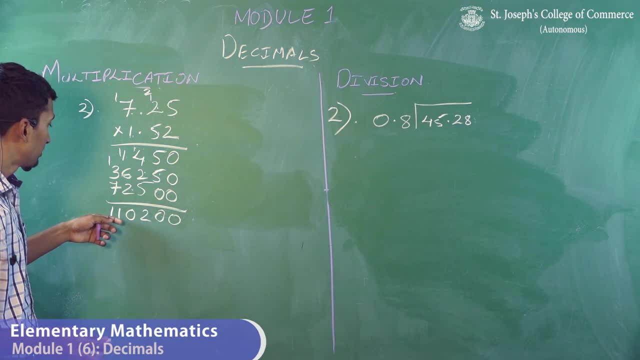 7 plus 3, 10 plus 1, 11.. Now you have double 1, 0, 200.. Now, over here, what we are going to do is we are going to go back and look at the decimal points. 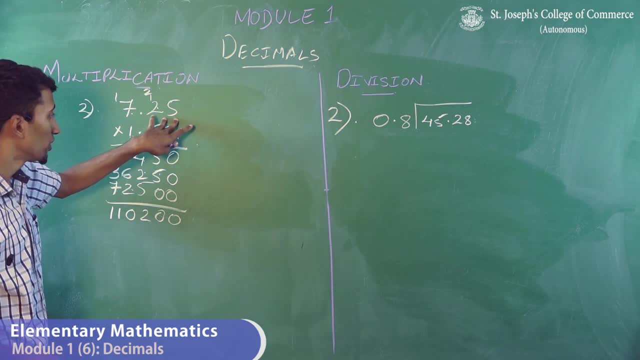 How many numbers are there after the decimal points? That is two numbers in the first and two numbers in the second. So that means four numbers totally are on the right-hand side of the decimal point. So over here we are going to. 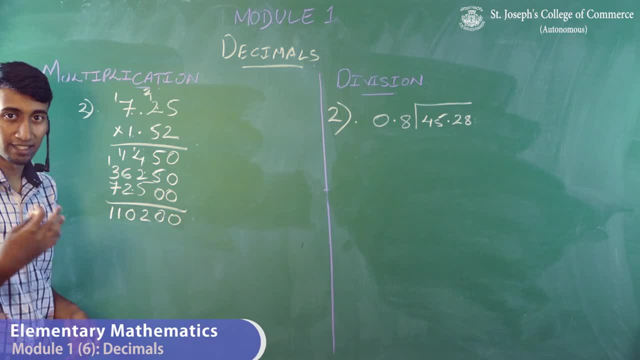 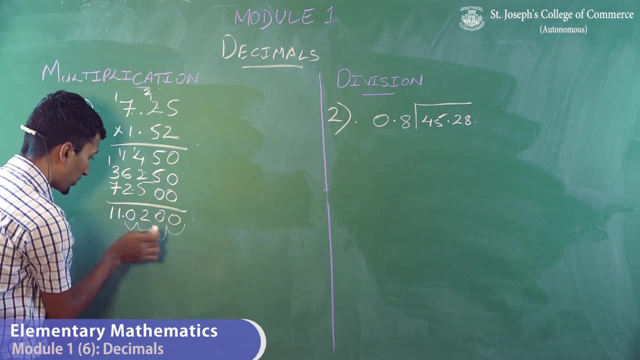 So that means I need four, Four numbers on the right-hand side of the decimal point. So I will just go 1, 2,, 3, 4.. So 11.02 is your answer. Now moving into division. 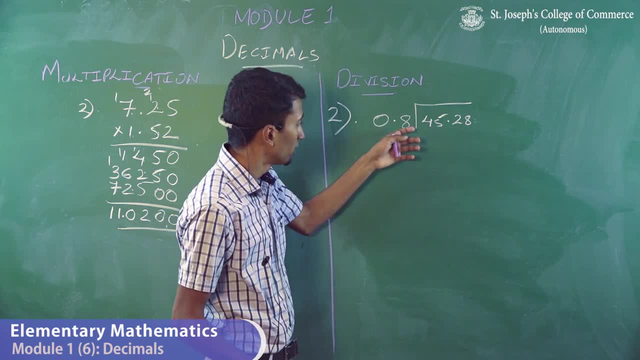 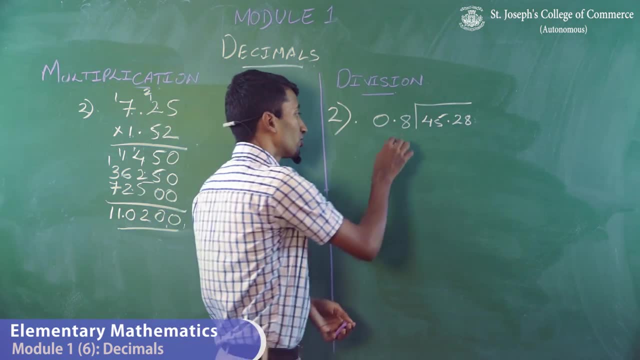 Now, over here it's 0.8 as your. Yeah, so 45.28 divided by 0.8.. So over here it's going to be a little tedious to solve the sum, So I just multiply this by 10 to make 0.8.. 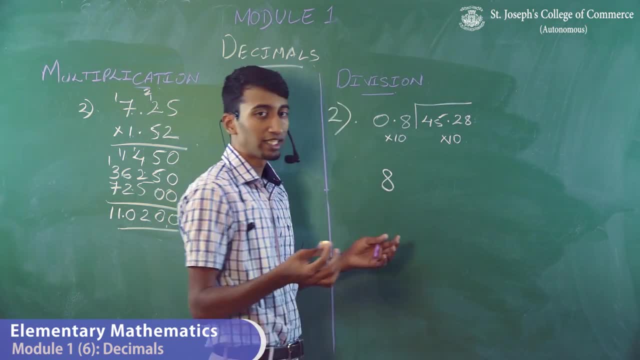 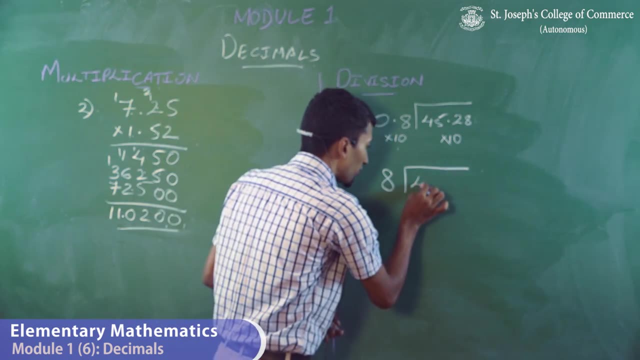 0.8 to 8,, which makes it much more easier. And so since I'm multiplying 0.8 by 10, I have to multiply this also by 10.. That would be 452.8.. Now, 8, 5 is a 40.. 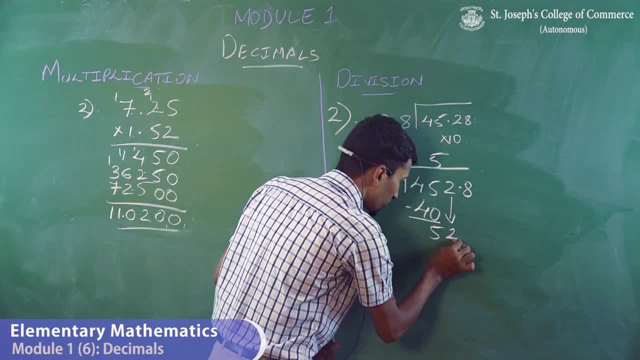 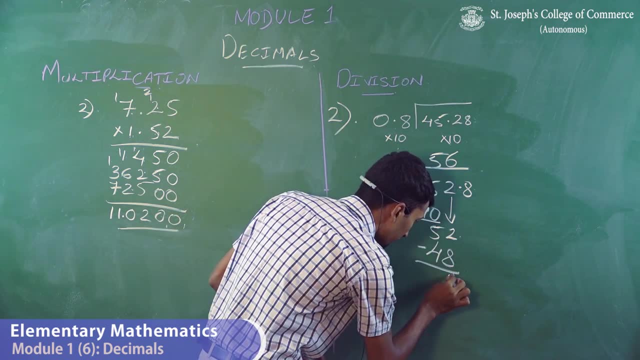 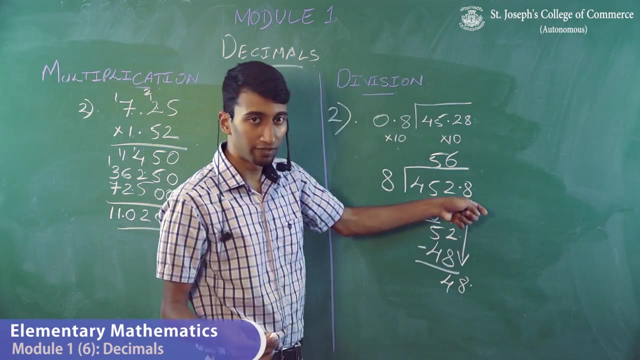 Minus, you get 5.. Get 2 down. So now 8, 6 are 48.. Minus and you get 4.. Now, get 8 down and you get 48.. Now, since 8 is after the decimal, so you have to put a decimal point. 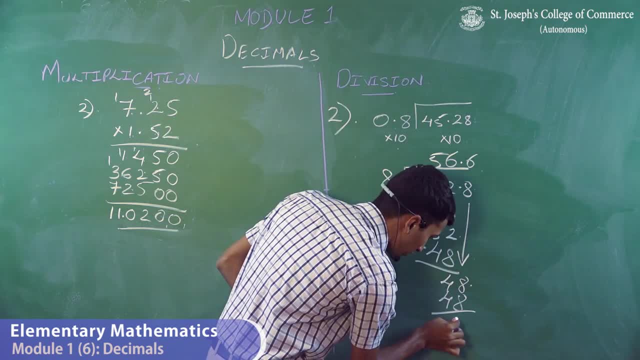 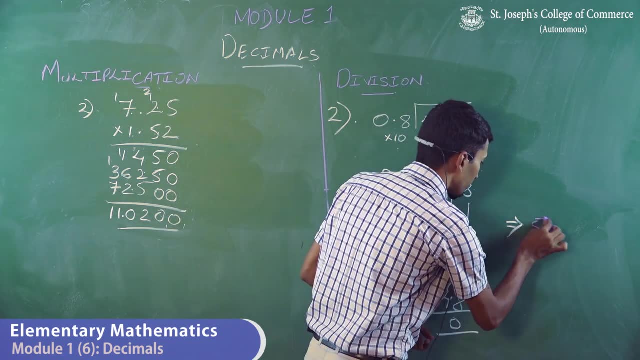 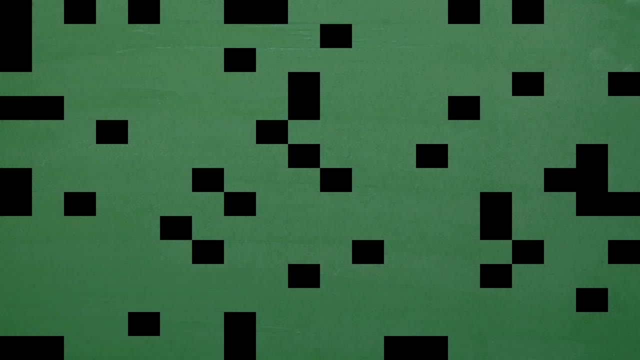 8,, 6 are 48, and you have no remainder, So this is your answer 56.6.. Thank you for watching. See you next time.